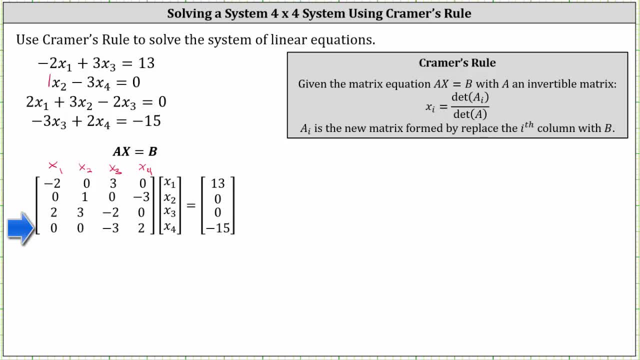 And then for the fourth equation, the coefficients of x sub one and x sub two are both zero. The coefficient of x sub three is negative three. The coefficient of x sub four is two. And then we have times, the variable matrix, where we have a column matrix. 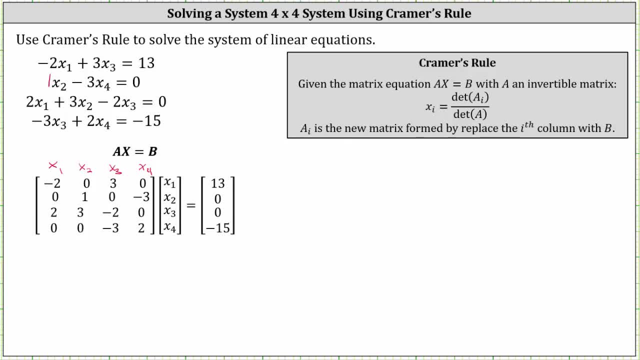 and the entries are x sub one through x sub four, equals on the right matrix B, which is a four by one matrix containing the constants on the right, We have 13,. zero, zero, negative, 15.. And now we can apply Cramer's rule. 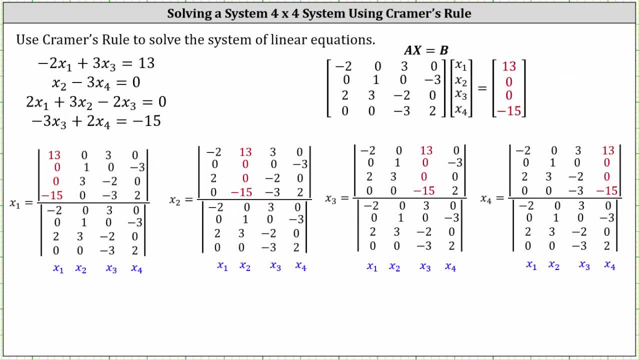 to solve for x sub one through x sub four. Notice: all the denominators for x sub one through x sub four are the same. We have the determinant of matrix A, the coefficient matrix, And now let's focus on the numerators For x sub one. the first column has been replaced. 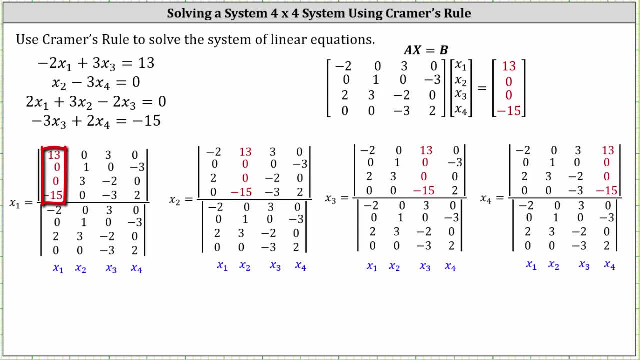 with matrix B, the constant matrix on the right, And columns two through. columns four remain the same. For x sub two, the second column is replaced with matrix B And columns one, three and four remain the same. For x sub three, the third column has been replaced. 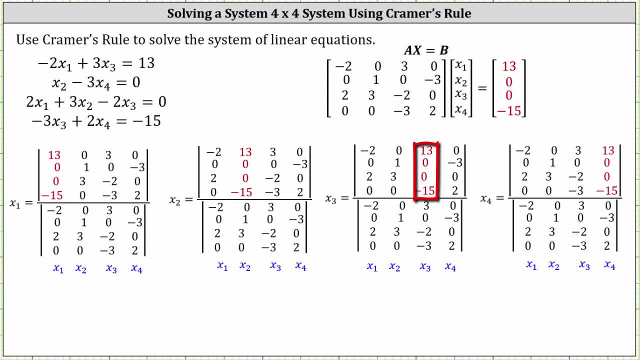 with matrix B or the constants on the right, And columns one, two and four remain the same, And for x sub four, the fourth column is replaced with matrix B or the constants, And columns one through three remain the same. 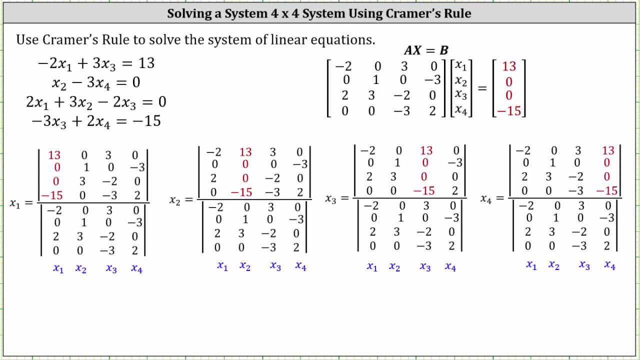 And now we just need to evaluate the determinants. And because these are four by four determinants, I already evaluated them with a calculator, where all four denominators are equal to negative 58 and the determinant of A sub one or the numerator of x sub one is equal to negative 106.. 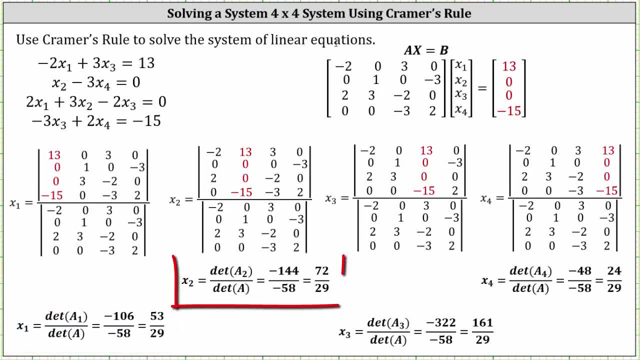 Simplifying we have: x sub one equals 53- 29ths. For x sub two, the determinant of A sub two in the numerator is equal to negative 144,. simplifying: x sub two is equal to 72 29ths. 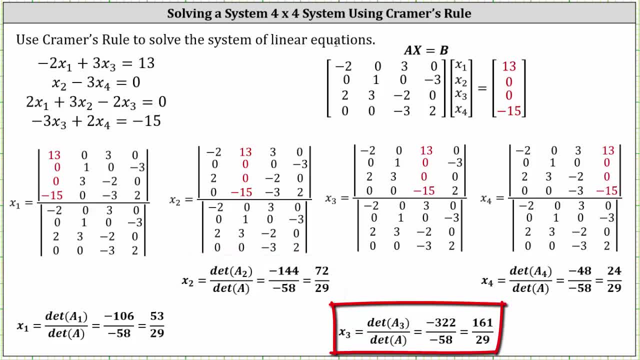 And for x sub three, the determinant of a sub three is equal to negative 322,. simplifying x sub three is equal to 161, 29ths. And finally, for x sub four, the determinant of a sub four is equal to negative 48,.